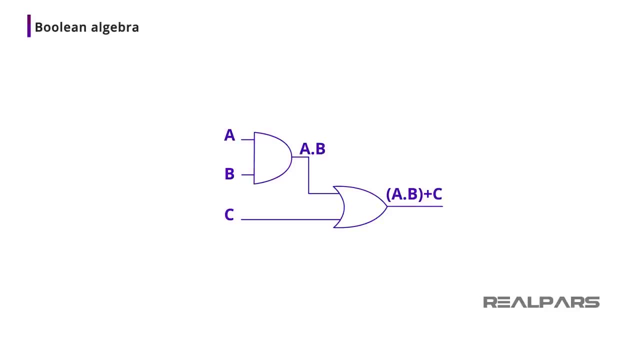 PLC programmers use Boolean algebra, also called Boolean logic, every time they create a program. Don't let the term algebra scare you, because the concepts of Boolean logic aren't terribly difficult. Boolean logic centers around the fundamental concept that all values are either true or false. 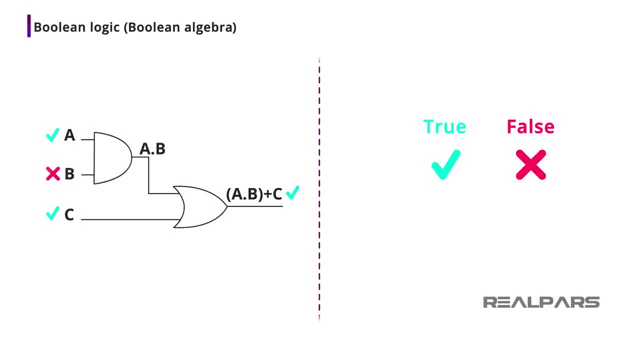 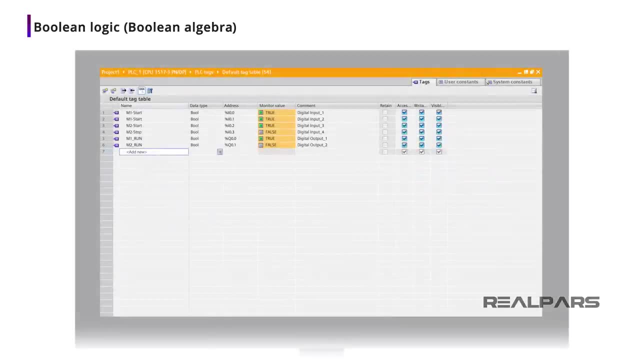 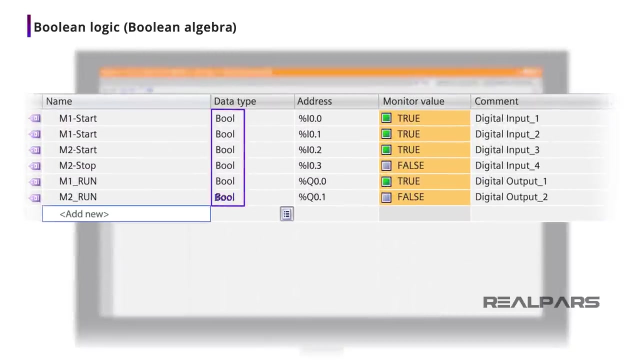 Going one step further. true and false can be represented by either a 1-bit or a 0-bit. You'll likely notice that most PLC programming languages use the term BOOL to represent a digital input or output. BOOL is short for Boolean. Every digital I-O can be represented by a 1 or a 0.. 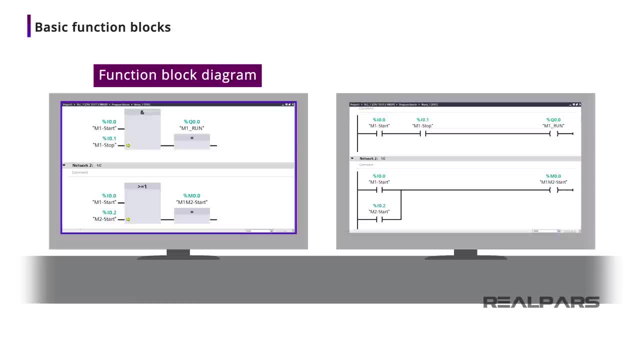 Function block diagram, or FBD, as described in IEC 61131-3, is rapidly replacing ladder logic as the programming language of BOOL is rapidly replacing ladder logic as the programming language of BOOL is rapidly replacing ladder logic as the programming language of BOOL. 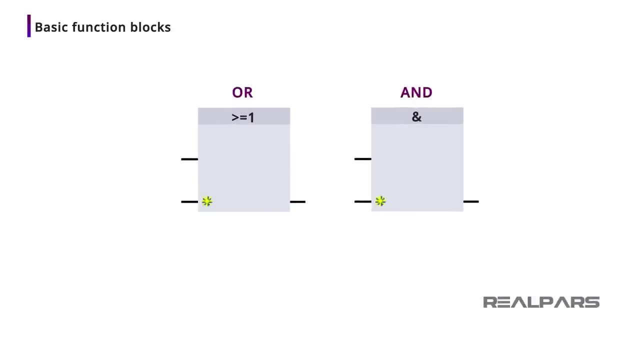 Let's look at the two basic function blocks in FBD and investigate the Boolean algebra associated with each. The OR function block has at least two inputs. Earlier we said in Boolean logic all values are either true or false and can be represented by either a 1 or a 0-bit. 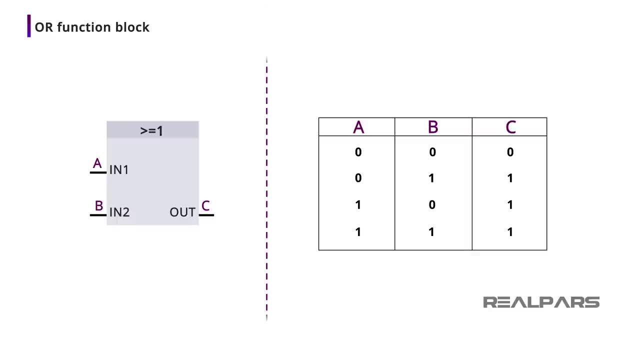 The OR function block has a truth table that does two things. First of all, it lays out all of the possible input conditions. Secondly, it indicates how the output reacts to the input conditions. From the truth table we can see that the C is true. 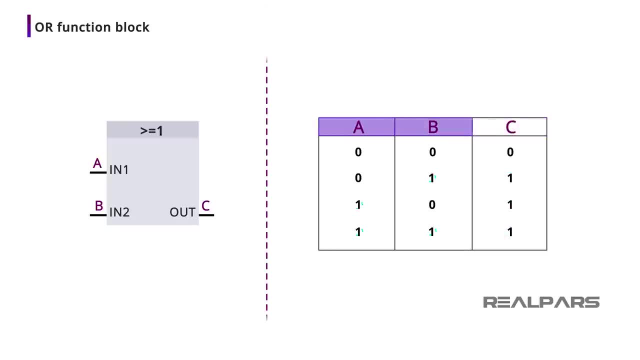 when A OR B is true. Okay, here's where we get into the Boolean algebra part. The mathematical expression for the OR function block is A OR B. OR B equals C. A plus sign is used to indicate the OR function. In primary school we were taught that the plus sign is used for addition. 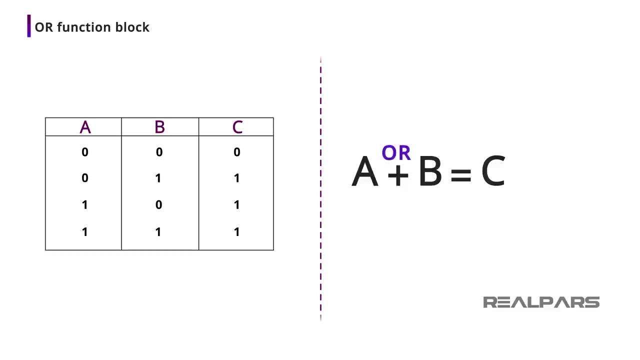 So it would appear that the OR function block performs Boolean addition. Okay, let's move on to the AND function block. The AND function block has at least two inputs. From the AND truth table we can see that C is true when A AND B are true. 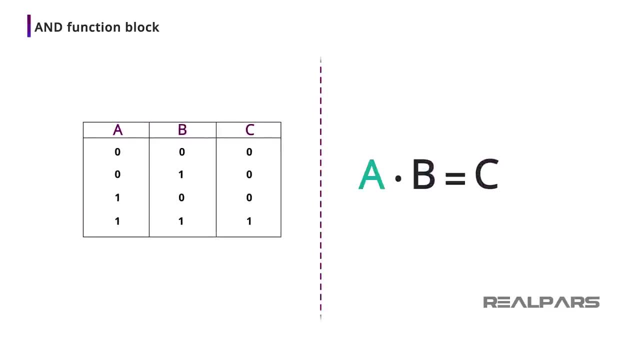 The mathematical expression for the AND function block is: A AND B equals C. Notice the multiplication symbol used to indicate the AND function. So it would appear that the AND function block performs Boolean multiplication. We can drop the multiplication symbol and the expression looks like this: 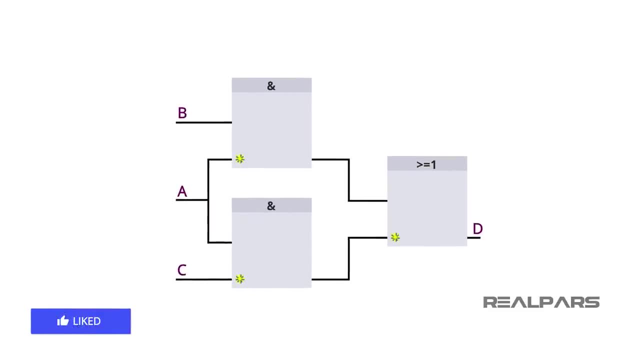 As we said earlier, PLC programmers rely on Boolean logic to optimize their designs. Let's look at a simple example of Boolean logic optimization. On the first pass of converting a system requirement into a function block diagram, a programmer ended with three function blocks. 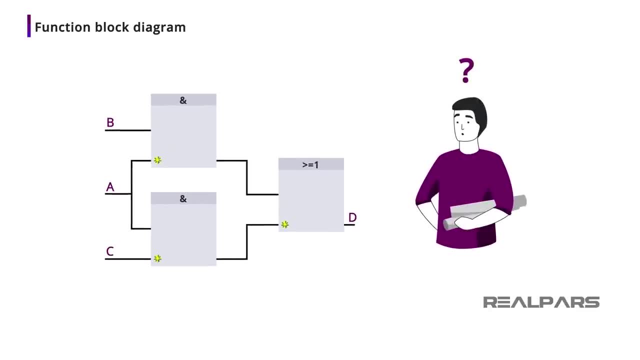 The programmer would ask herself: Can I optimize this function block diagram and eliminate any of the function blocks using Boolean algebra? The answer is yes. So let's see how The Boolean logic expression for this program is. D is equal to AB plus AC. 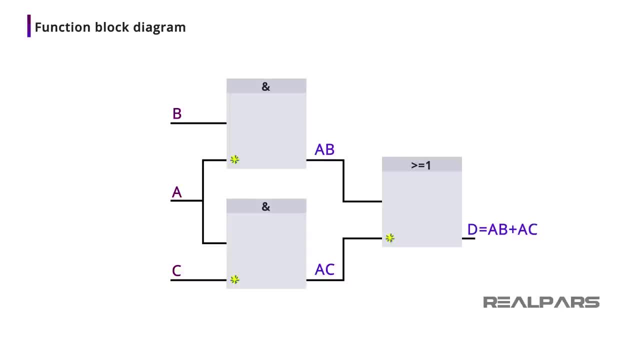 Using a little high school math. we use the distributive law and a transformation occurs. Alright, now let's rebuild our function block diagram and see if we've made some progress toward optimization. After using some basic algebra, we've gone from three function blocks. 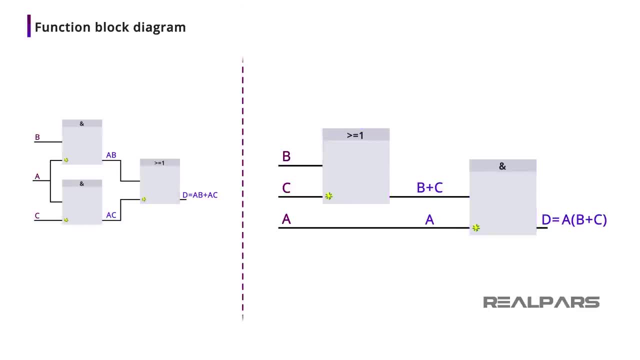 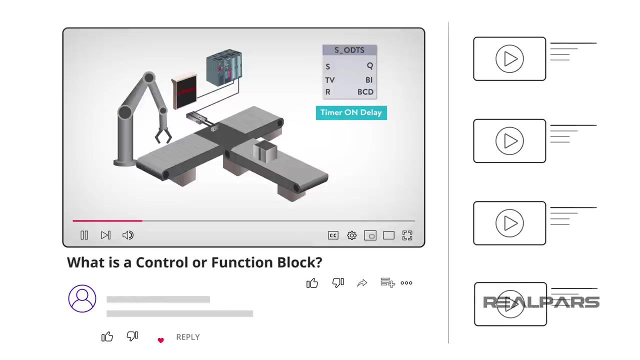 to two function blocks. We've given you just a glimpse of how Boolean logic can be used in the optimization of PLC programs. Like it or not, seasoned PLC programmers have become mathematicians. If you want to learn more, you might want to review two of our other videos called. 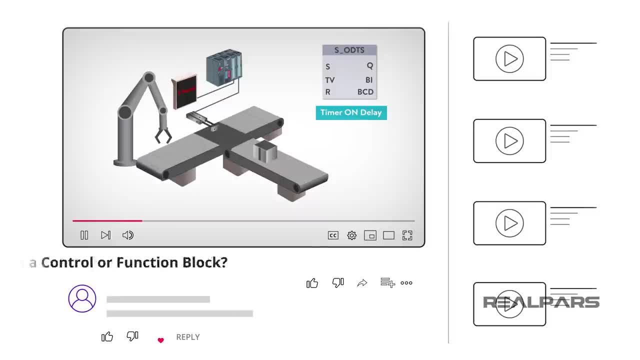 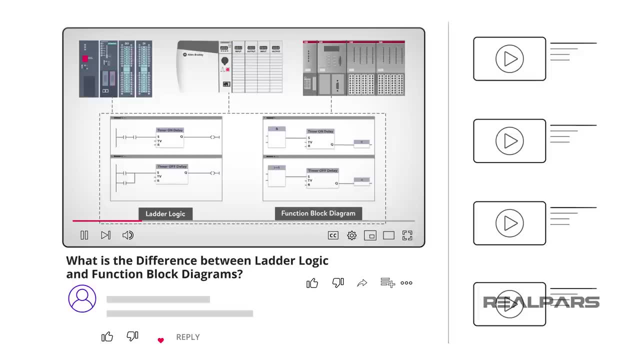 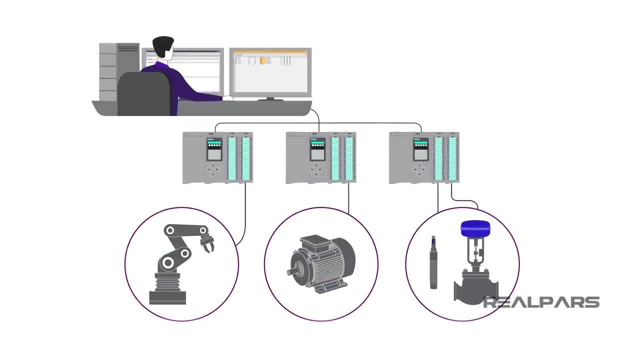 What is a control or function block and What is the difference between ladder logic and function block diagrams? You can find the links to these videos in the description. Ok, let's review what we've covered in this video. PLC programmers possess a variety of knowledge and skills.